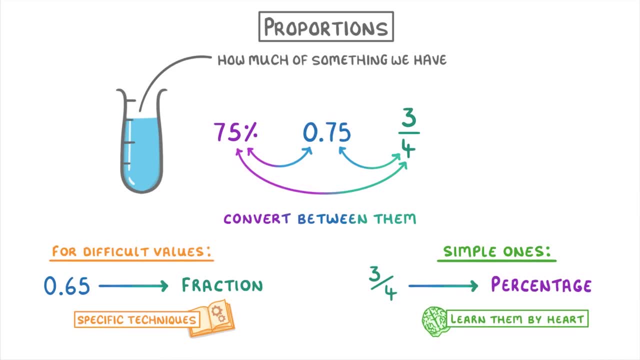 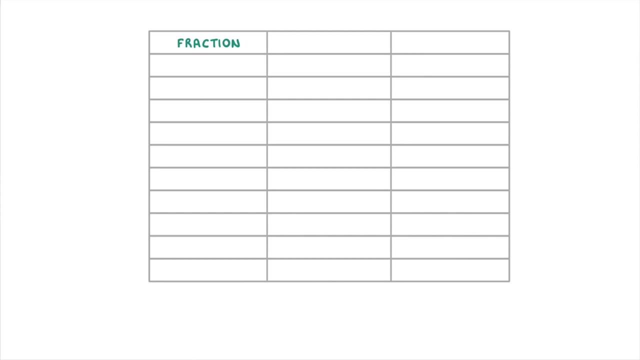 it's much easier if you just learn them all off by heart. So for the rest of this video we're going to go through the most common ones that are worth memorising. The best way to do this is to make a table with fraction, decimal and number. You can use any number. 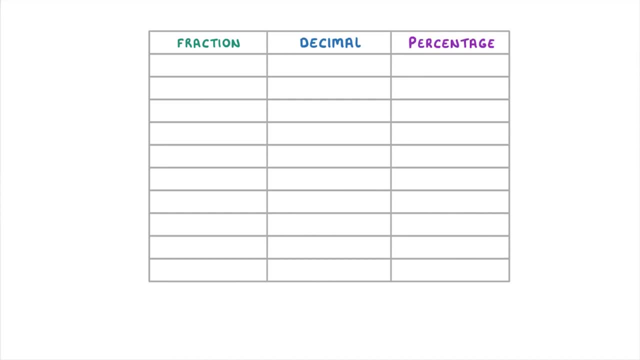 you like, and you can also use the number you want. If we start with 1 over 10,, that would be equivalent to 0.1, or 10%, Whereas if we had 2 over 10, that would be equivalent. 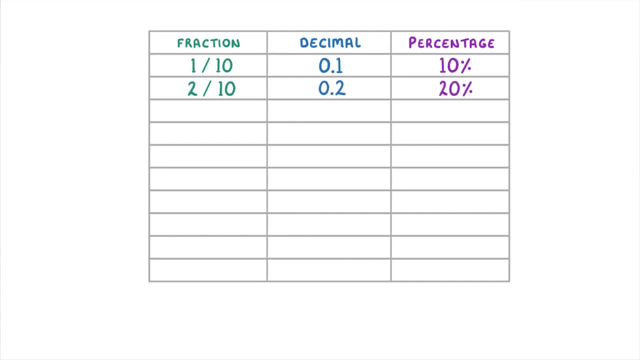 to 0.2, or 20%, So everything is just 2 times as big. And we could keep on going like this all the way up to 1 whole, which is 100%. Now, instead of trying to memorise this entire table, it's much better for you to just remember. 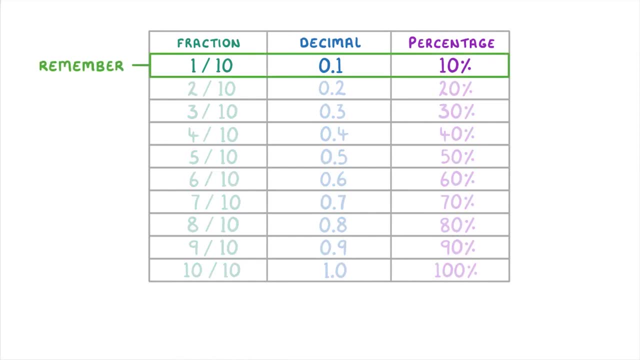 the first row and then understand the pattern so that you can work out all the others. One thing you need to watch out for, though, is the simplified versions of fractions. For example, 2 over 10 is the same thing as 1 over 5.. So one fifth is equivalent to 0.2,. 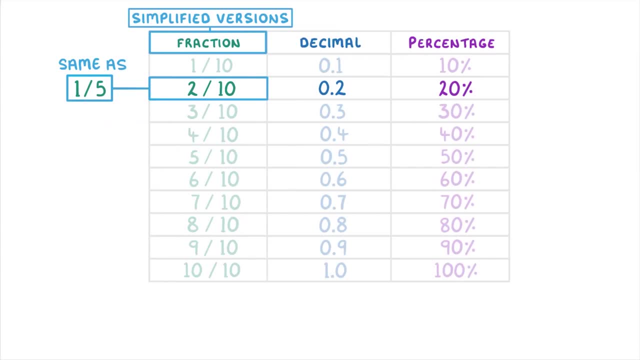 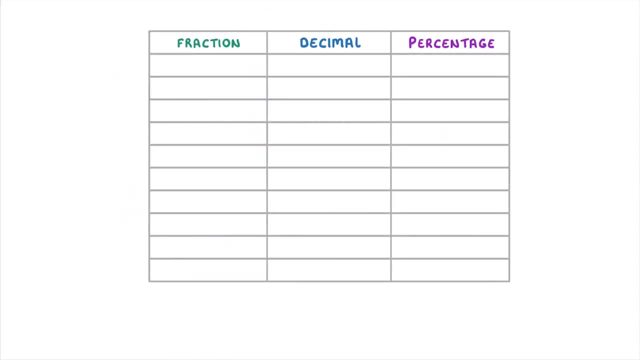 and 20%, And the same goes for these other simplified versions. We're not going to go through all of them one by one, but just so that you've seen them all, it's also worth knowing one half, one third, one quarter, one fifth and one eighth. 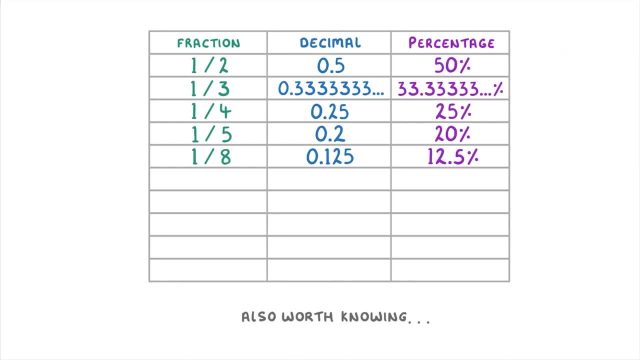 And if you know all of these, then you can generally work out most of the other ones that you might need. For example, if we wanted to find out what 3 over 8 is equal to, then it would just be 3 times as much as 1 over 8.. So 0.375 as a decimal or 37.5% as a percentage. 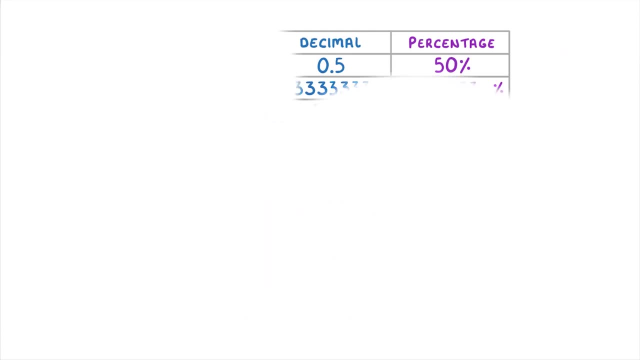 Anyways, that's everything for this video, So if you enjoyed it, then do give us a like and subscribe And we'll see you next time. Subtitles by the Amaraorg community.